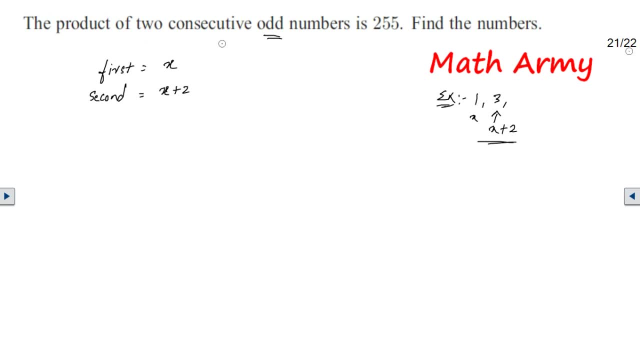 applied here right Now. same logic applies to even numbers as well. Now what they are saying: the product of x and x plus 2 is equal to 255.. So write that Now. multiply x with x plus 2.. So x square plus 2x equal to 255.. Now bring 255 to the left hand. 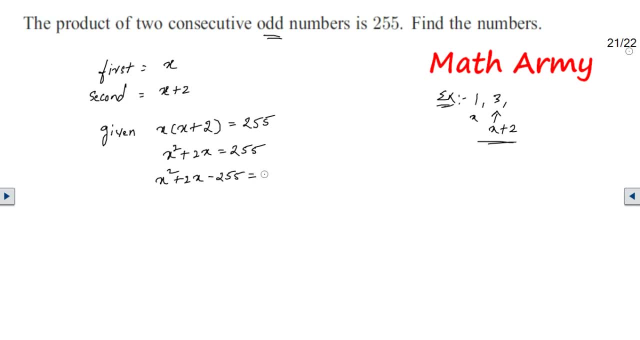 side It becomes minus 255.. Now it is looking like a proper quadratic equation for me. Now split the middle term in such a way that the product should be minus 255 x square and the sum should be plus 2x. So what are those two? 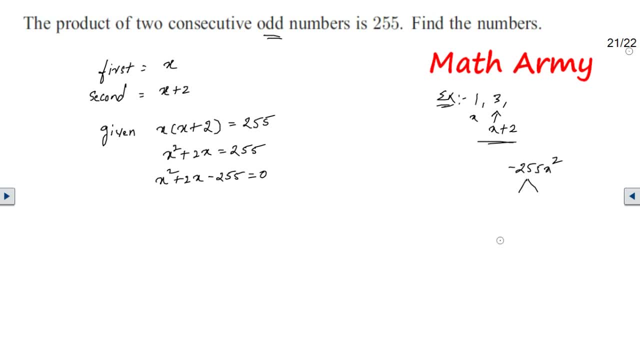 numbers. Guys, if you are really good at tables it is fine. Otherwise you know 15, 15 tens are 150 and 15 sevens are 784.. So let me check with 15 first. I think I should be able to get that I am dividing 15.. Sorry. 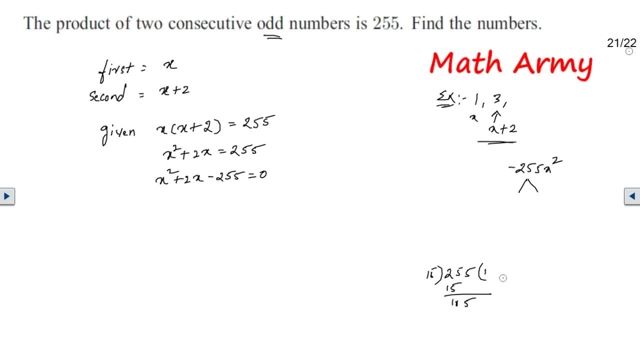 255 with 15.. 15 ones are 15, 10, bring down 5 and 15 divides 105 in 7 times Now. yes, Now the difference between 15 and 17 is 2.. So, because I need plus 2, so I am going to put plus. 17 here. So I am going to put plus 7 here. So because I need plus 2, so I am going to put plus 15 and I am dividing 15.. So this is minus 15.. And then I'm adding 15 to the middle term. I'm 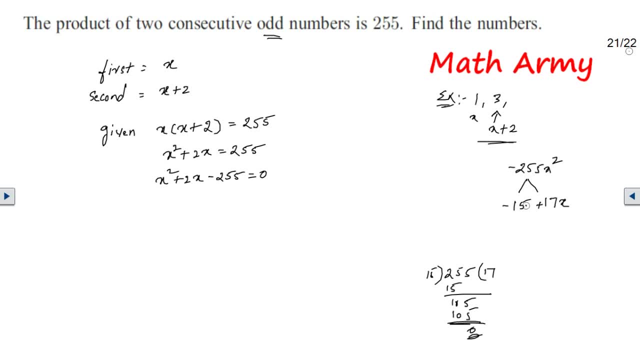 17 and minus 15x, right? So that is how this is going to satisfy my condition for factorization. So write x square, as is. instead of plus 2x, you can write minus 15x and plus 17x. 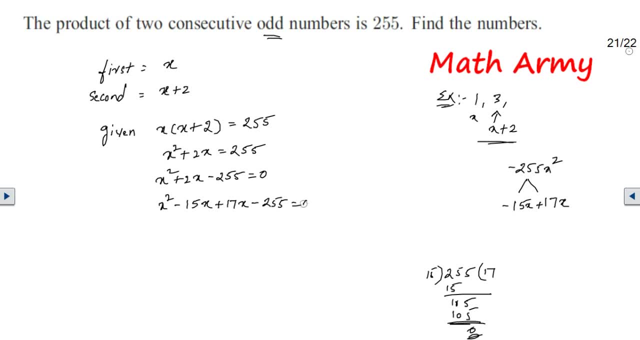 and minus 255, equal to 0. Now, between the first two terms, what is common? See, guys, if you add them you are going to get plus 2x right Now take x common- x minus 15 is the first factor. Now take plus 17- common- x minus 15 is the factor.